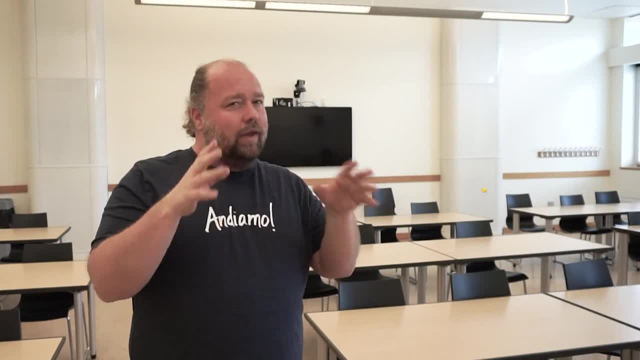 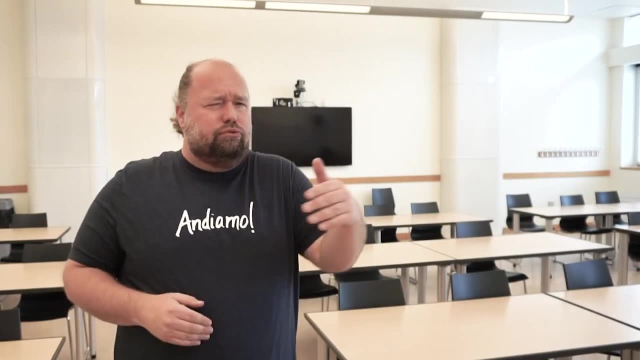 about it in general: in our promotion strategy, What role will advertising play? Is it gonna be a big part or a small part? Because we have movies, right, You do have all the commercials and the pre-roll ads on YouTube and stuff like that. 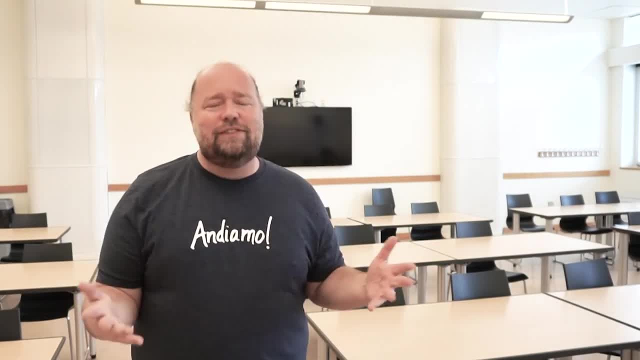 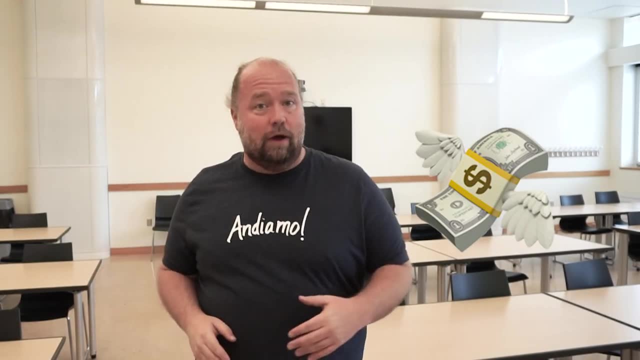 I mean, heck, I'm sure you probably saw a pre-roll ad on YouTube or some movie before this video. And the thing is you see that, look, we have those advertising things, But also we've got to pay for the actors to show up for the world premiere. 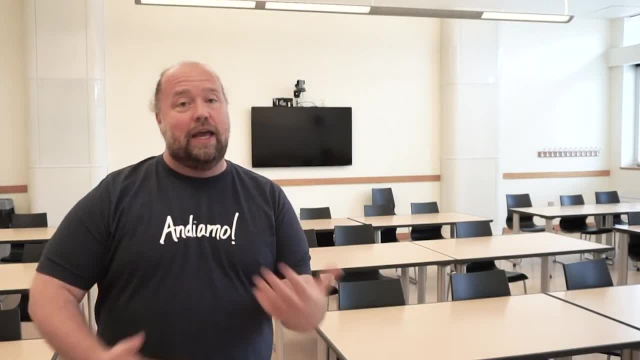 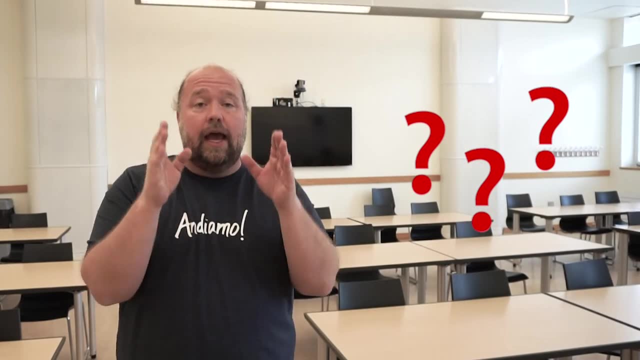 in Hollywood and the world premiere in Shanghai, right, And so we have all those things. So there's all kinds of different ways we promote. But we really got to figure out is: what is advertising's role? Is it to get people excited? Is it gonna be a? 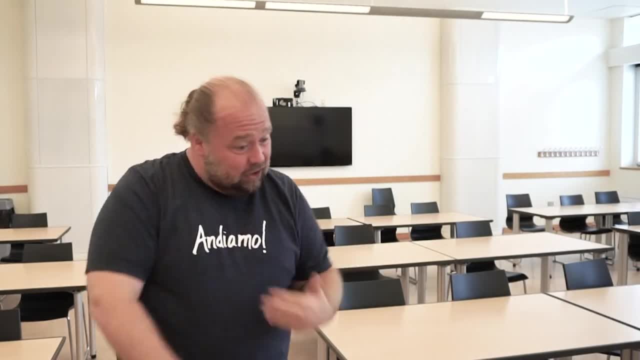 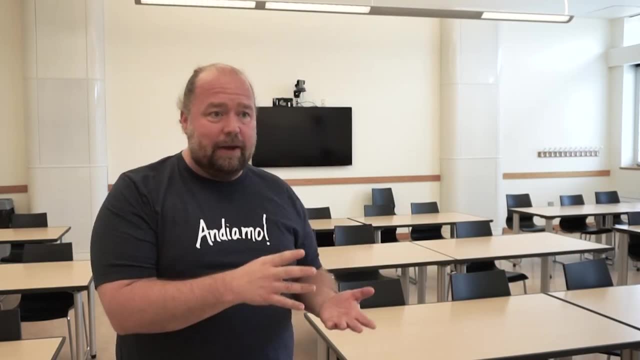 big part, a small part, whatever, like that, And that's why we have to look at. our next step is: how big of a role is it going to play? Okay, what role is it going to be Then? how big is that part going to be When you think about it? are we going all in on? 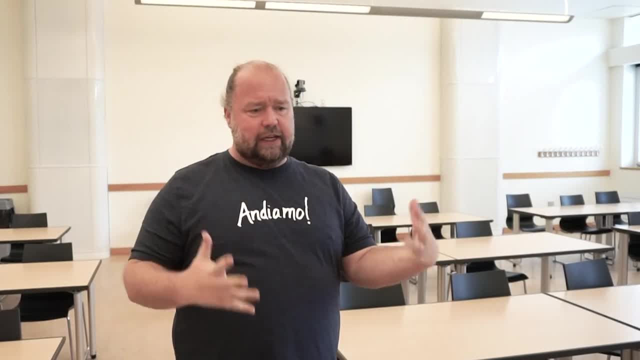 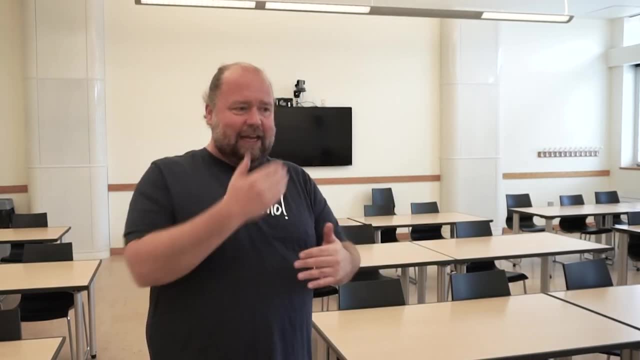 a Super Bowl spot. we're going to spend four or $5 million to this 30 seconds to get people to know, Or are we going to spend, you know, a few hundred thousand dollars and have thousands of 15 second videos playing in front of YouTube videos? Well, a. 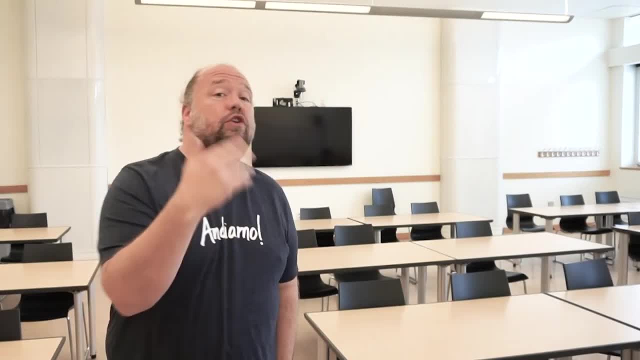 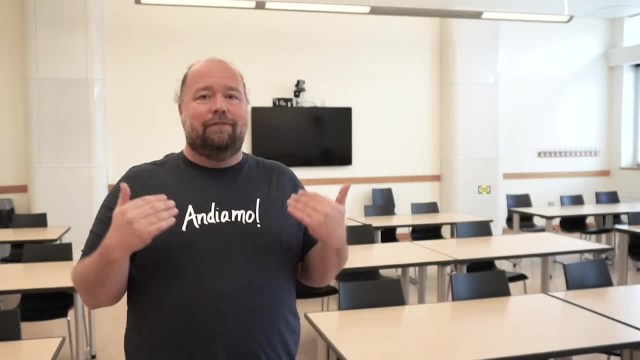 lot of it will depend how important that audience is that you want to hit And so by doing that, that really influences what are advertising budgets going to be? Because, look, if I'm a nonprofit- I am not- I don't have the money. Let me check. 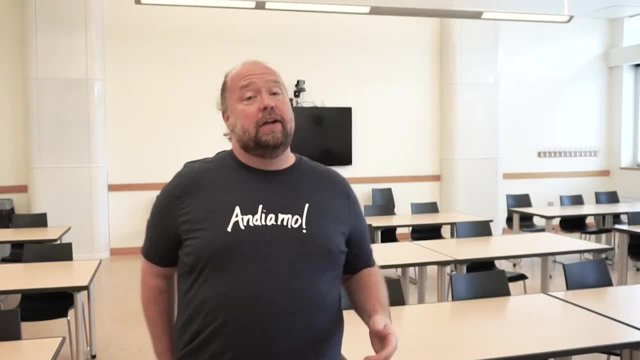 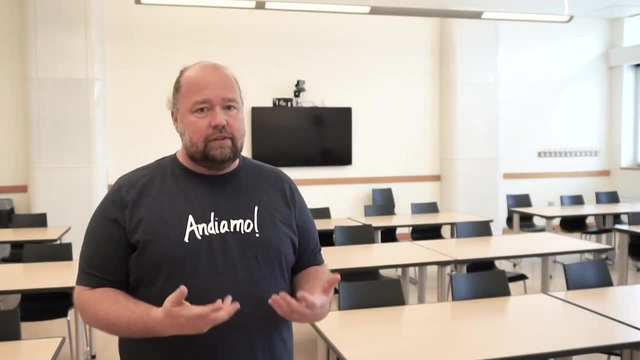 Yep, I don't have the money for a Super Bowl ad, But a nonprofit. they might be able to spend a few hundred dollars here and there to put out some Facebook ads or Instagram ads and stuff like that. So we start to see like, look, if we're going to have a. 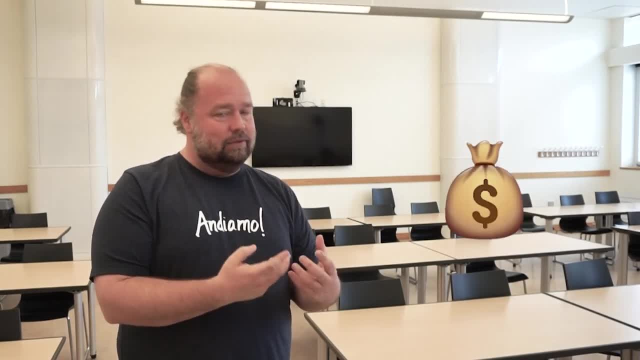 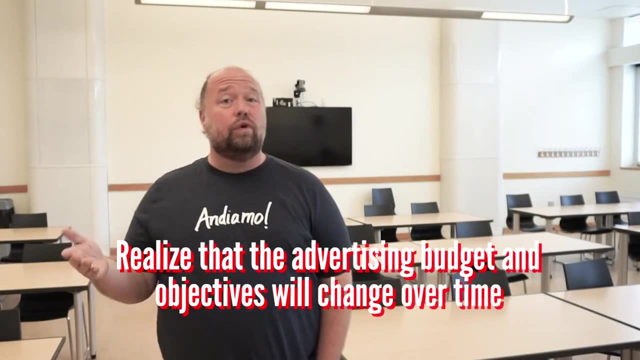 big role here. it's gonna need a lot of money And we don't have a lot of money. Well, that's going to influence it, right? So we have to think about these things And what you have to realize is your advertising budget will change over time, Because think, 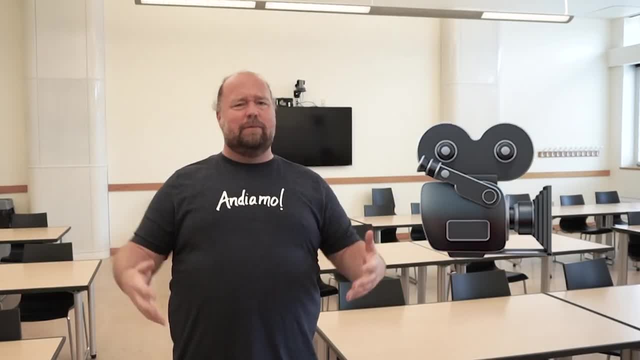 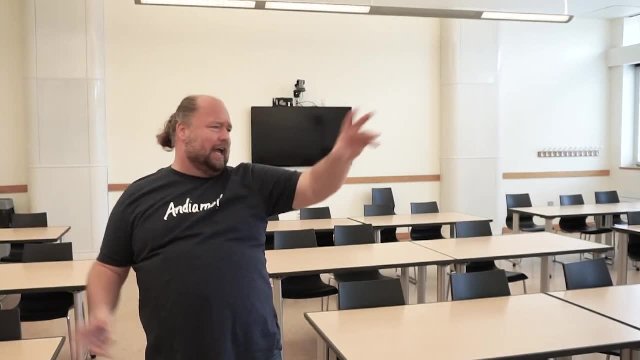 about it when a new product comes out. let's think about movies. right, A new movie is coming. you see tons and tons of commercials for it. right, Coming this May, the new Avengers movie. oh, you got book tickets now. all tickets on sale now. 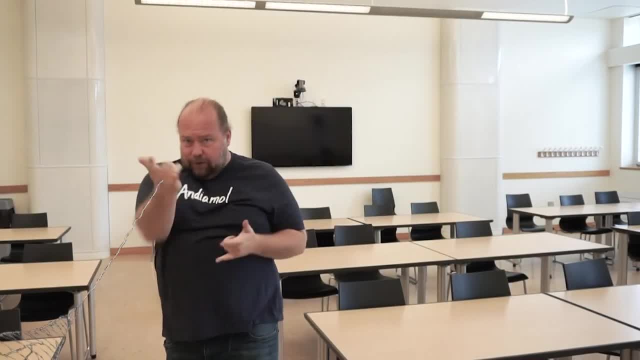 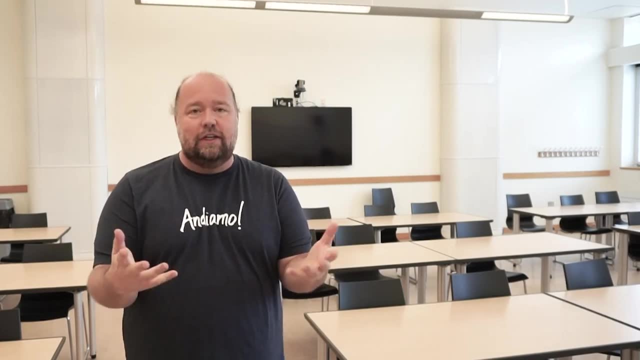 And they show like whatever superhero is popular now going through there and Spider-Man's gonna be back and all this kind of stuff, And people get all excited, right, Because they're commercial, commercial, commercial because we're introducing it, We're letting people know the thing is coming. 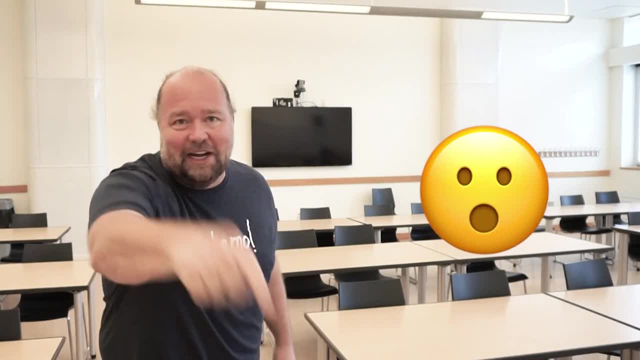 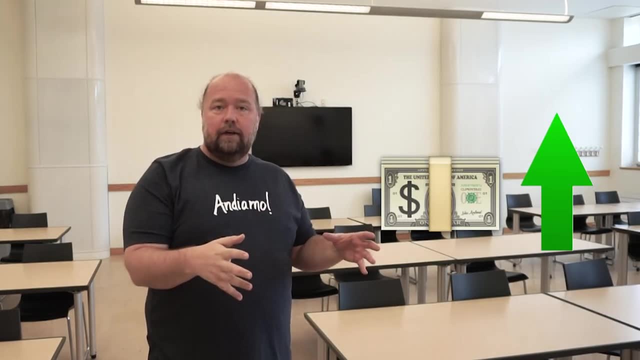 out. People got to get people excited. We got people to know that this new movie is coming, And so we're our budget for before, or advertising budget before the movie comes out, is gonna be a lot higher than after it comes out. I mean think. about it. You hear all the ads, all the commercials, see all the stuff online before the movie comes out through the first weekend, And then all of a sudden you notice it starts dying off. You're like: wait, why am I not getting like 1900? 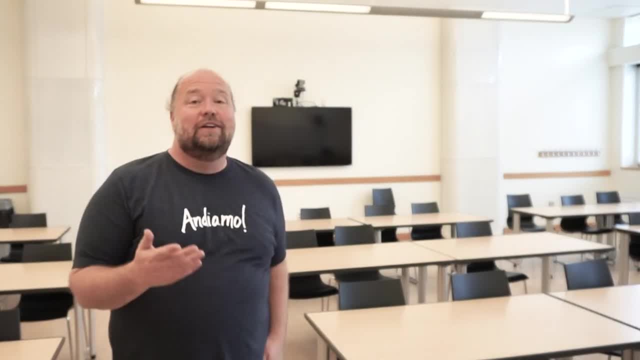 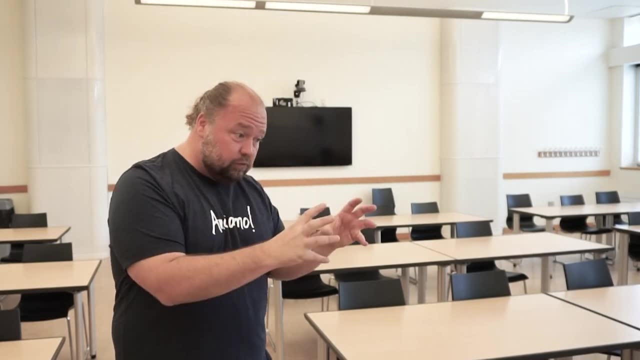 Avengers ads or something like that. What's going on here? Well, what you end up doing is you start seeing- is that you actually the budget switches because we have this big push to get people to go to the movie theater that first weekend. 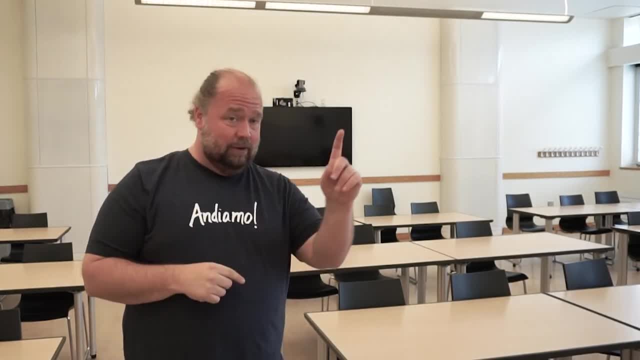 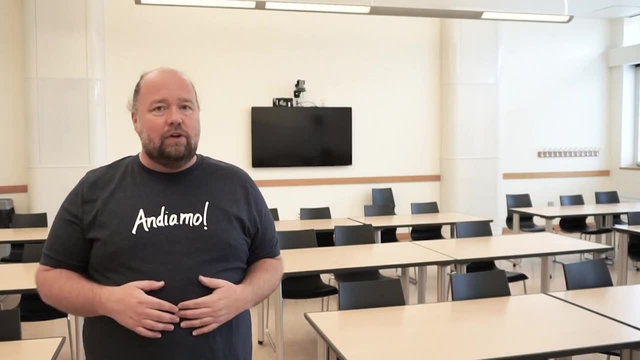 because we know we've got to be the number one movie in America or the number one movie in the world. Because then the next time we're moving on later into the growth phase, we're looking at in terms: of: look, we're not trying to educate people, not. 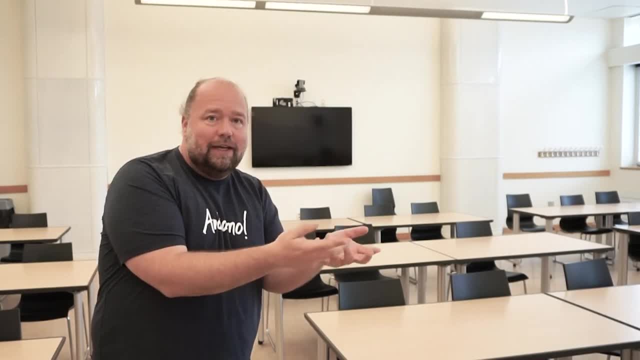 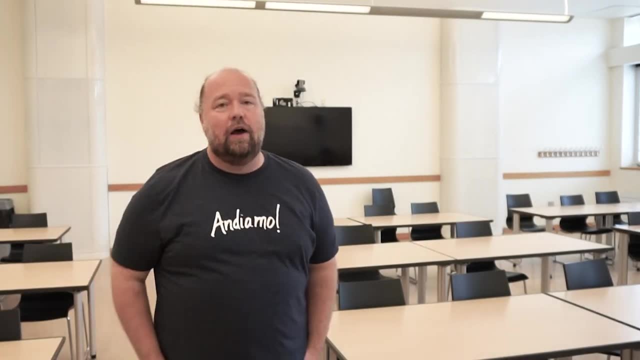 trying to inform people about what our product is like. we do in the introduction phase, In this growth phase. Now we're telling people: hey look, you should come see our movie instead of the competition. Hence, why at the first weekend if it's the 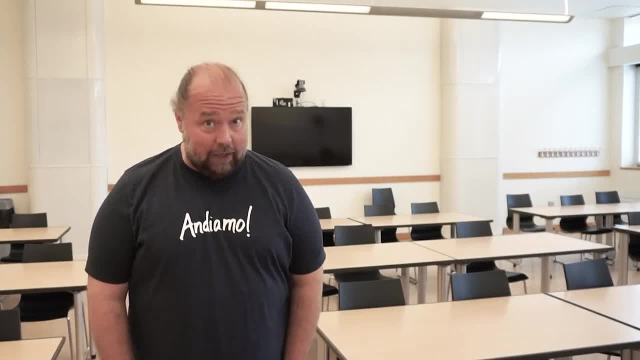 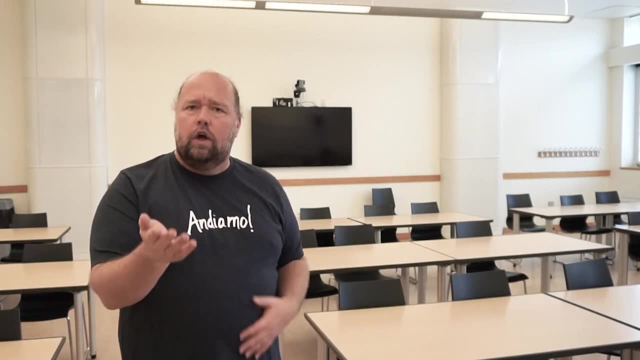 number one movie in America. you darn well know their advertisers will be the number one movie in America, right? And so you have that. And so what we're trying to do is to get people to just persuade. oh, you're not sure what movie to go to. Well, everyone else in. 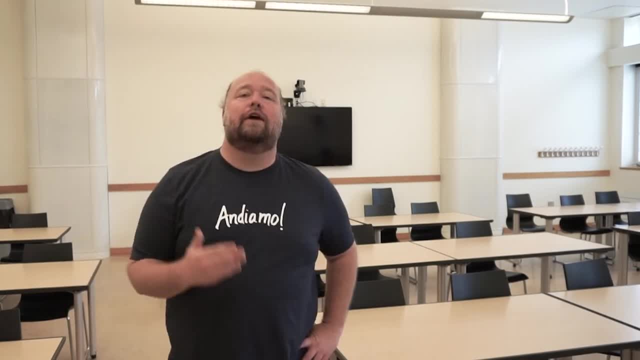 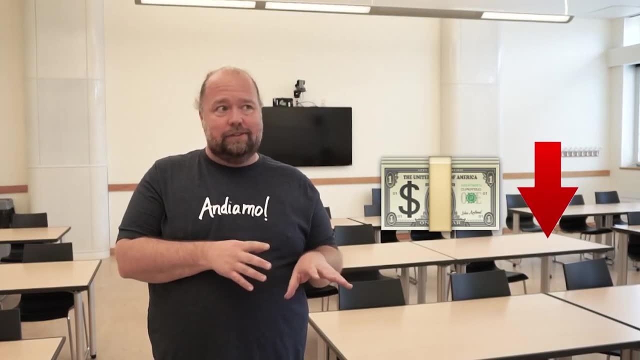 America last weekend went, saw this, So shouldn't you see it as well? So they're trying to persuade you, trying to give you a reason to do that. And the thing is is during this growth phase we're spending less money on our advertising because 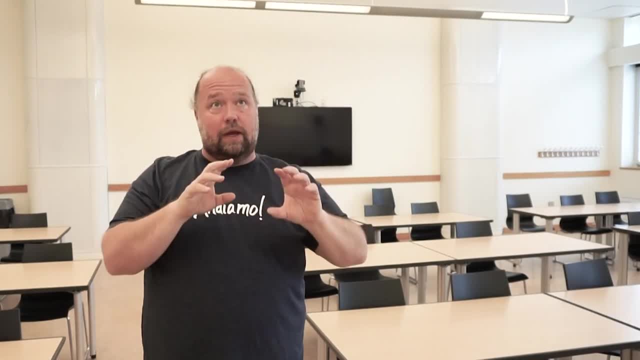 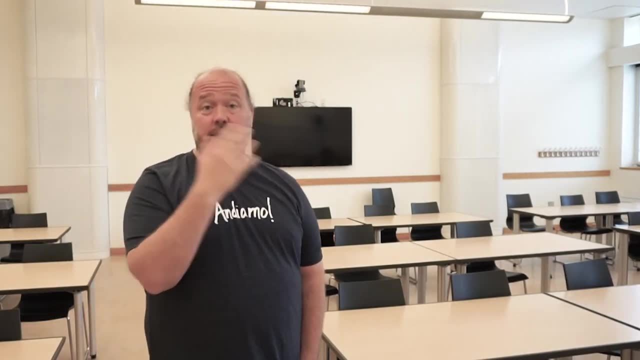 we're not trying to get the word out. The word is already out. People are nowhere there. Now we're just trying to persuade people to buy from us And we have all that residual memory from those like lots and lots of ads In the introduction phase that we kind of play a little bit off. 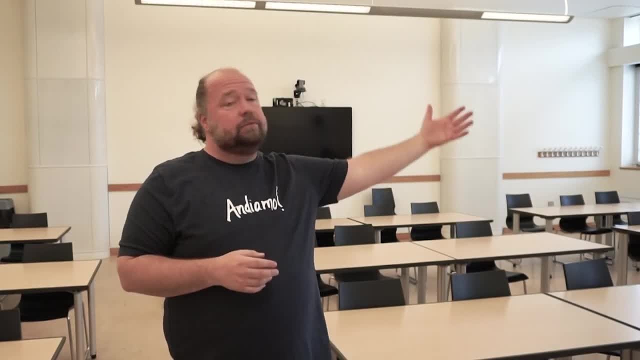 of that, because you know what you remember: ads from days before, weeks before, months before. there's still a little bit in there, So we don't have to advertise it quite as much Now. we're just focused on specific things. Look, if you're looking. 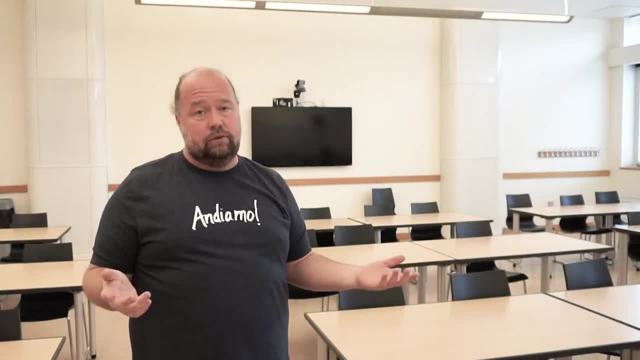 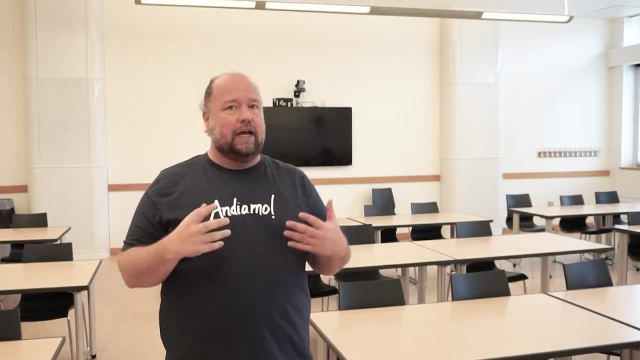 for the most fun movie, go see this. I don't have to educate you as much, Okay, And the thing is, if you're looking at your budget, as you go farther down that product lifecycle, if you're getting into the maturity phase, I mean, think about it, there's. 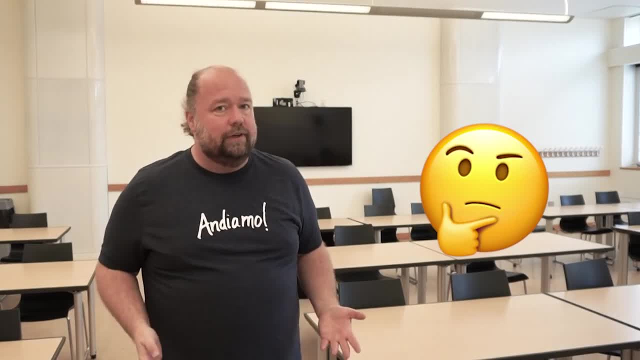 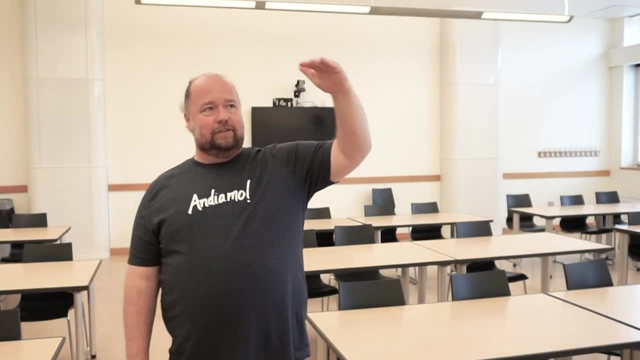 not a lot of new people going out to buy that product. What are we doing? that maturity phase? we're just trying to remind people, hey, see that Avengers movie again and you'll see like the number of ads for movies it's like super high at the. you know the. 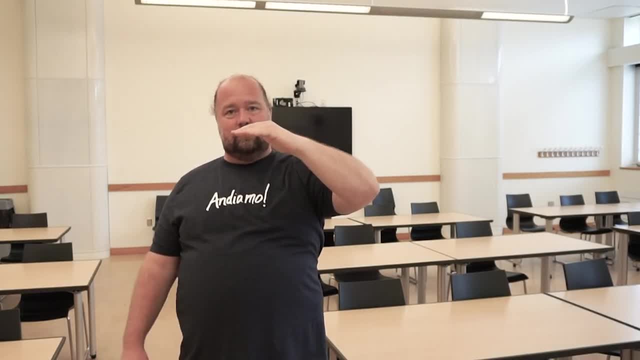 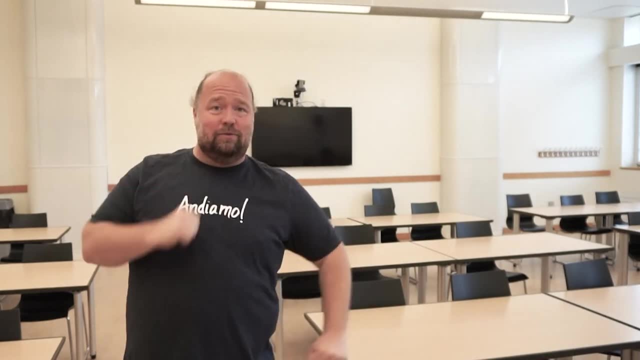 weeks leading up the movie, And then it's like here after the movie comes out, and then like two weeks out, you see, like no ads, no commercials, maybe a few billboards and occasional- Hey, why not go and take another spin with Spider Man? you know they. 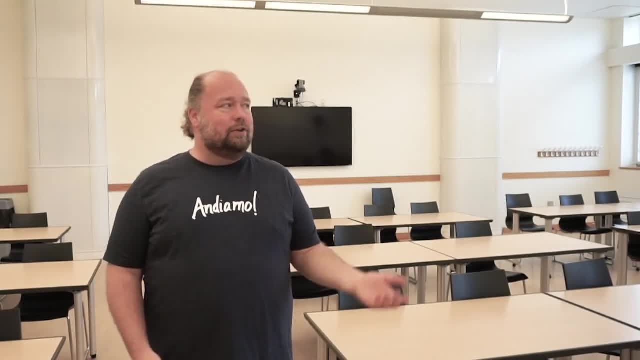 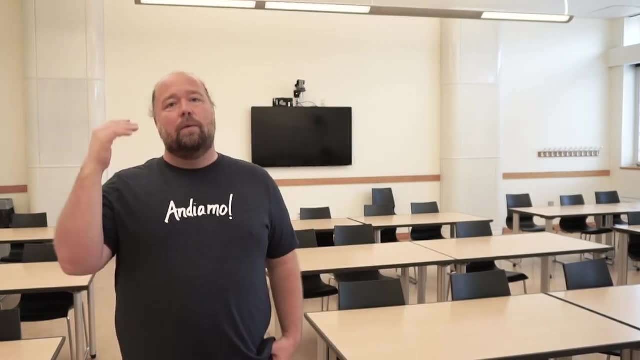 do that because they realize the maturity phase. everyone already knows about the product. what I'm really doing is that reminder advertising, just like, hey, if you haven't seen yet, why don't you go check it out? And so doing that, you start to see is you're going to have different. 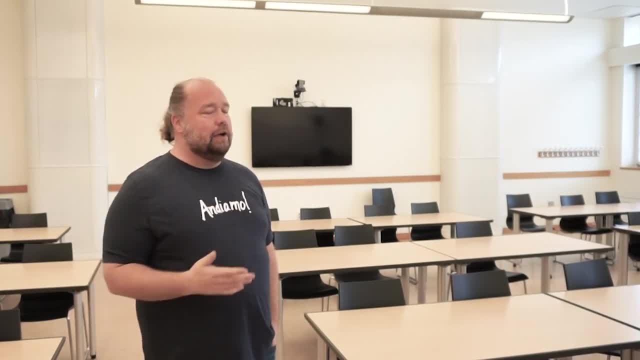 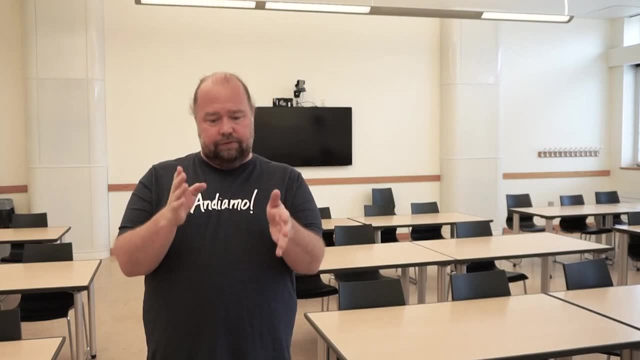 budgets for different time periods, And so when you're making and you're determining your advertising budget, you might plan it out. This is our advertising budget for the before the movie comes out. Here's our advertising budget budget for the three first three or four weeks the movie's. 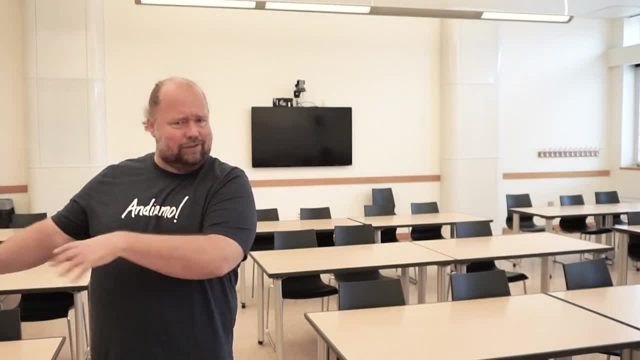 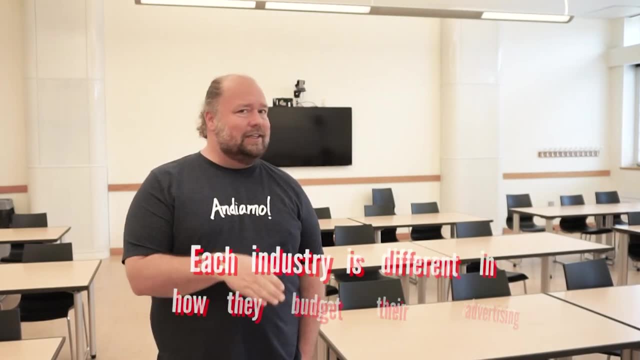 out. And then here's our advertising budget afterwards made for the DVD release or something like that, right, And so you kind of have different plans out there for your budget, And what you have to realize is each industry is different when it comes to advertising. like you know, I've got my 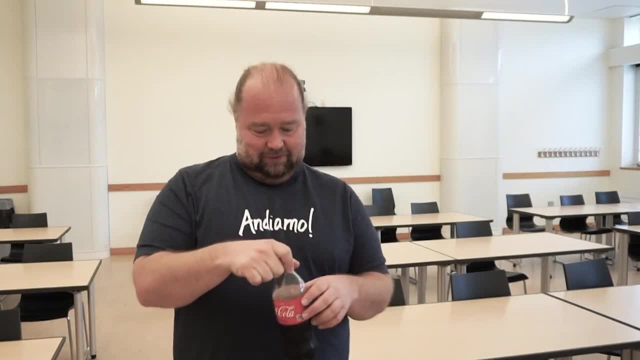 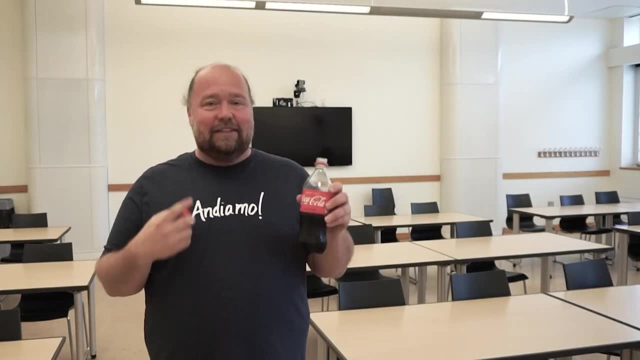 budget here, Because after filming like 25 videos- if you ever noticed the last exam, I'm wearing this Andiamo shirt a lot. That's because I'm filming a lot at one time. And the thing is Coke. you see a lot of advertisers for Coca Cola. But 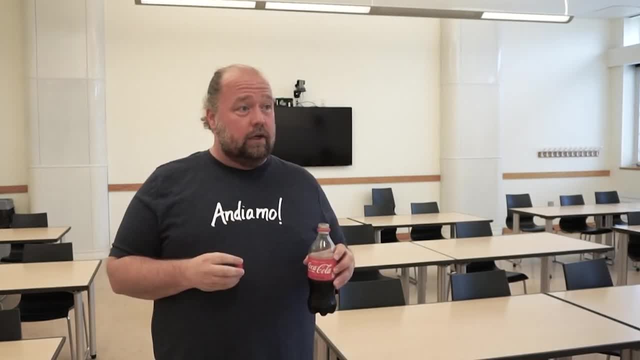 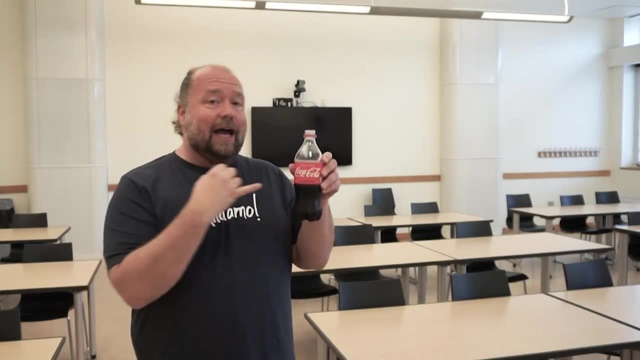 do you see many ads for cinnamon Coke? Do you see many for you know, cherry vanilla Coke or cherry Coke by itself? Not so much Because in the cola industry they know that. look, I can advertise this beautiful, wonderful, original taste Coca. 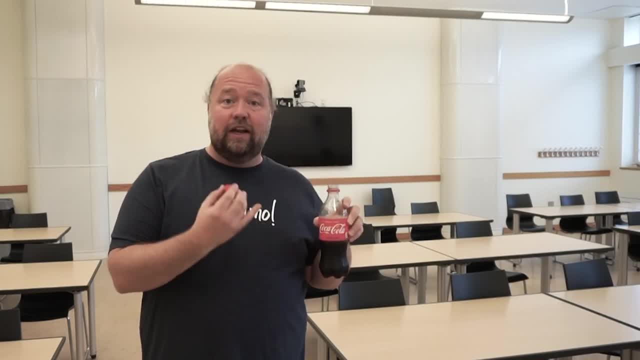 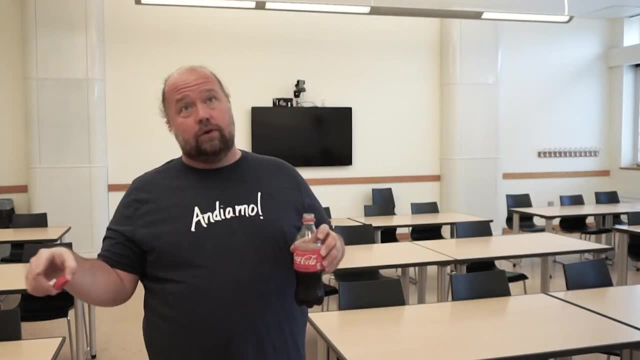 Cola And it still kind of works like I'm advertising for: Diet Coke, Coke Zero, cherry Coke, cinnamon Coke, cherry vanilla Coke, orange vanilla Coke, orange Coke, Coke with lime, Coke with lemon, caffeine free Coke with lime or lemon. right, You have all those. 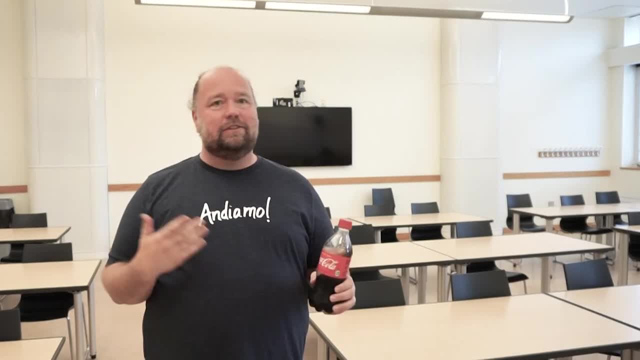 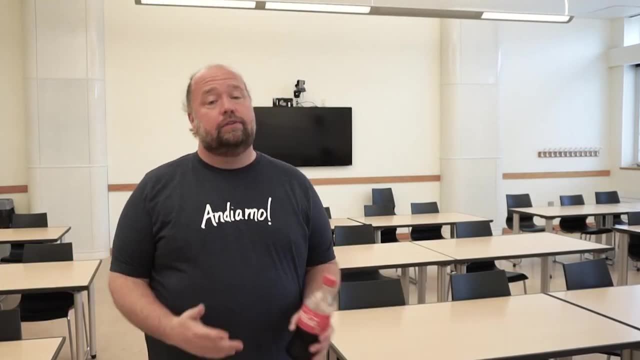 things out there. And so you see that you have to realize, look, our advertising budget is going to be different depending on the product we have, what we're trying to do. the different spot it is the lifecycle. So you have to consider all those things. 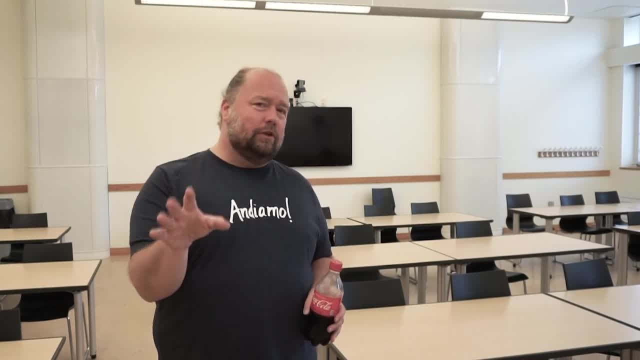 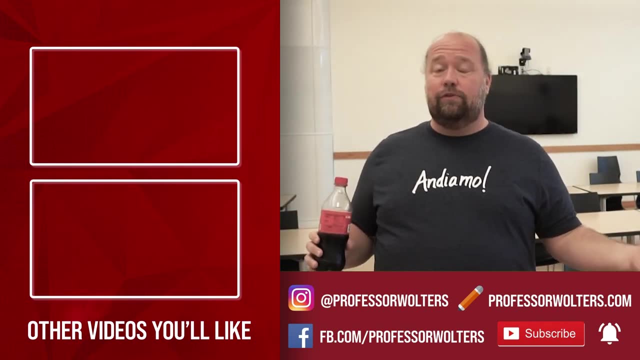 when you're determining your advertising budget. Okay, so I hope this helps you understand a little bit more about this advertising campaign and planning for our advertising campaign. Remember there's other steps out there you got to go through, So watch those videos whether you're looking. 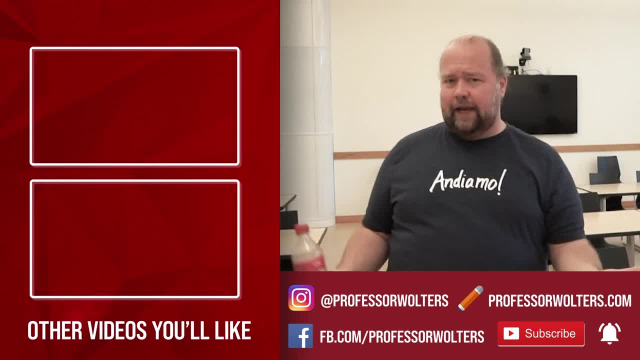 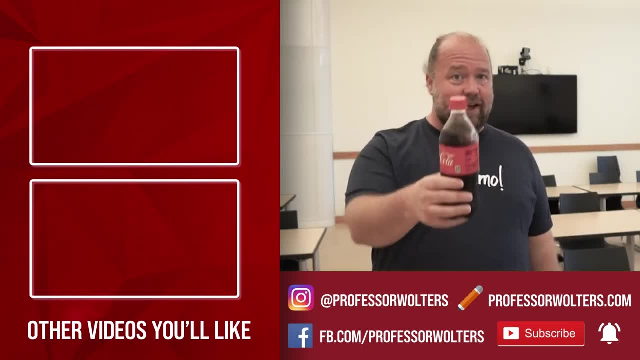 at how to decide who to target with your ads, how to set objectives for your ads, maybe assessing the impact of those ads or how good they could work. We have videos on those two. So good luck and I'll talk to you later.